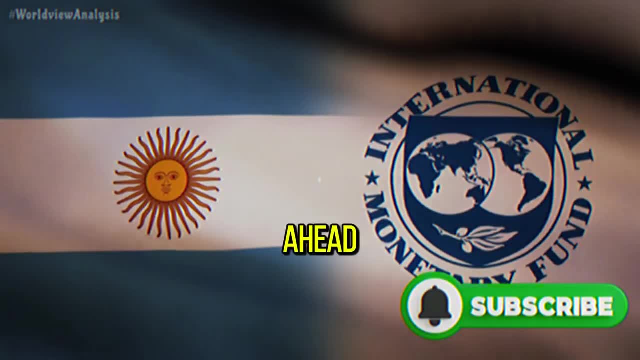 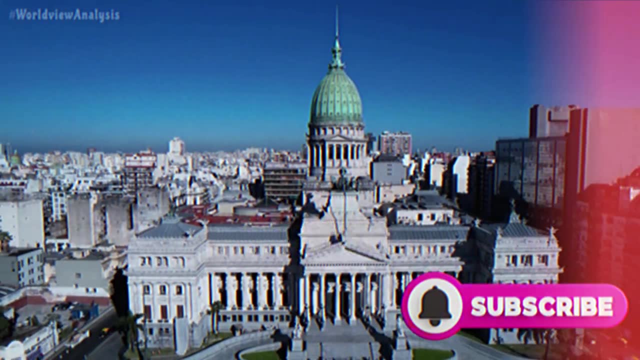 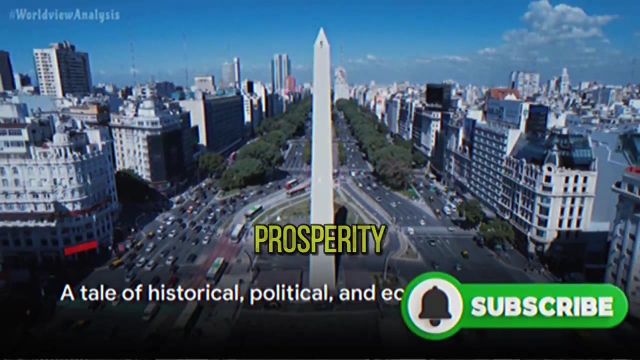 and growth, there were signs of the challenges that lay ahead. Economic inequalities rooted in the country's colonial past persisted, and the reliance on a few key sectors for economic growth made the country vulnerable to global market fluctuations From this pinnacle of prosperity. 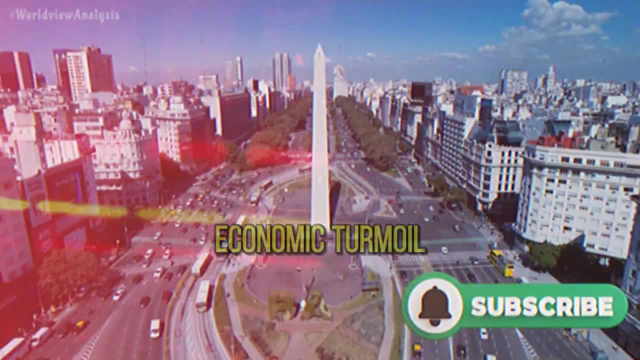 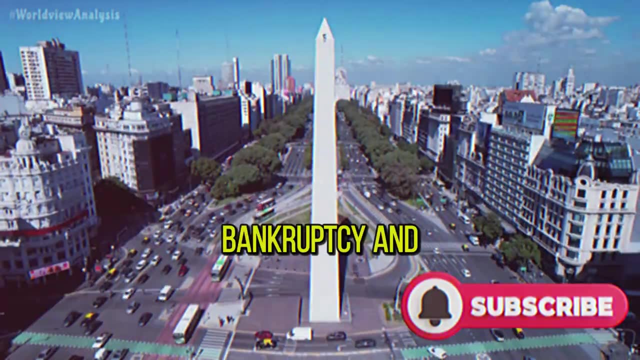 it's hard to imagine Argentina's forthcoming descent into economic turmoil, As we'll see in the following scenes, the journey from economic giant to a nation struggling with bankruptcy and social unrest is a complex tale of historical, political and economic dynamics. For now, let's 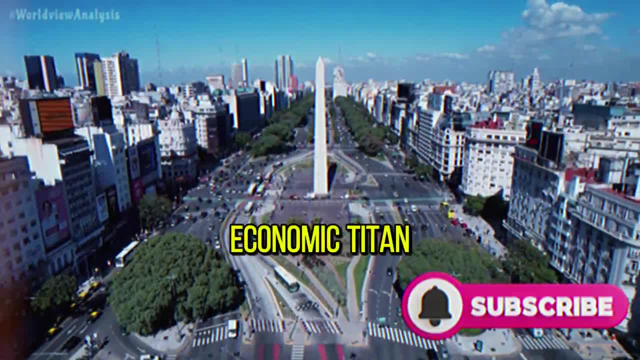 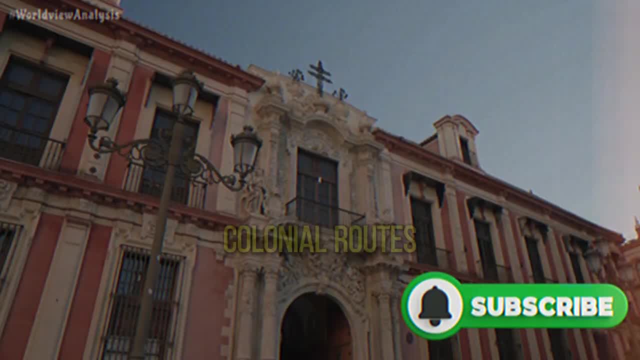 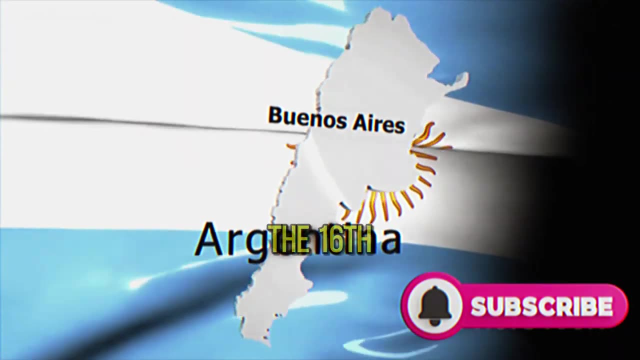 pause and reflect on the rise of Argentina, once an economic titan standing tall on the global stage. To understand Argentina's economic journey, we must travel back to its colonial roots, to the Spanish settlements, in pursuit of silver. The labyrinth of history leads us back to the 16th. 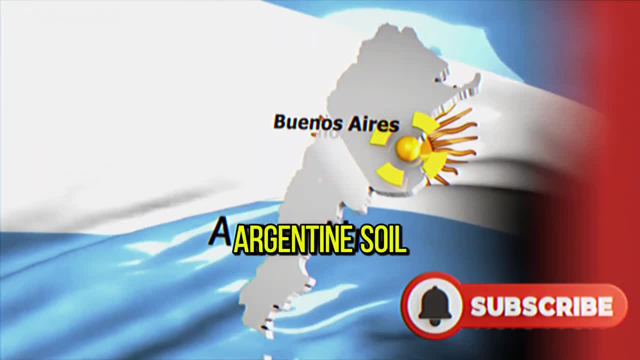 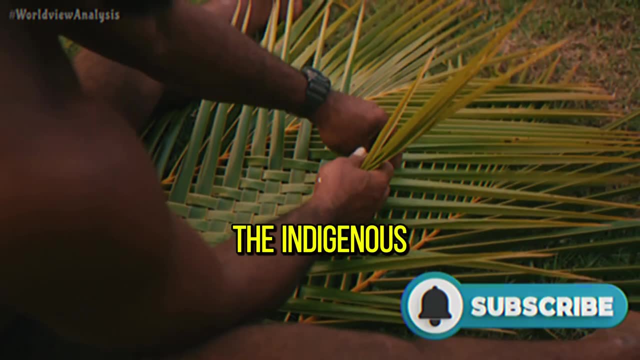 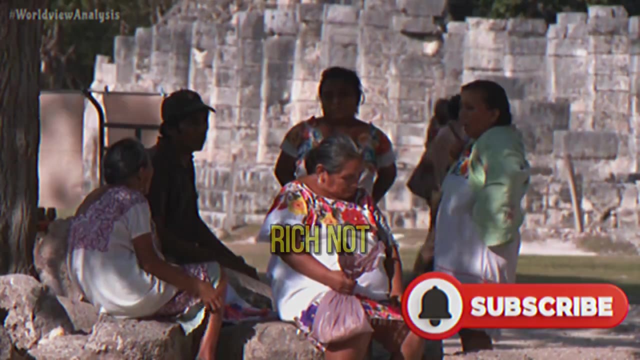 century, when the Spanish explorers landed on Argentine soil driven by their thirst for silver riches, Their dreams of prosperity were intertwined with the fate of the indigenous people, whose labor and resources were exploited to fuel Spain's economic ambitions. The Argentine soil was rich, not just. 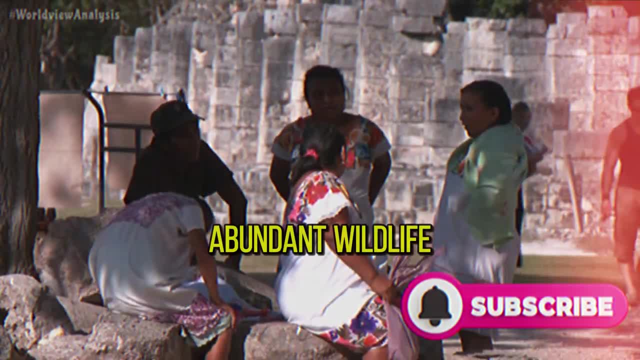 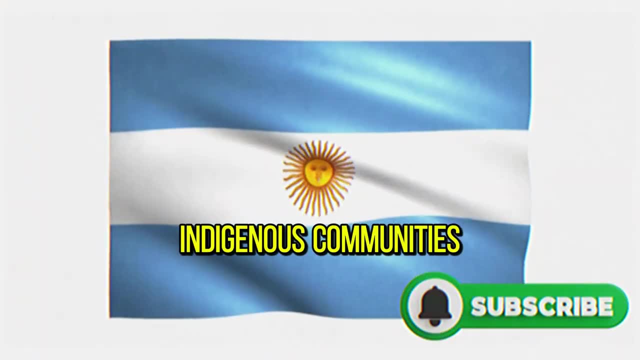 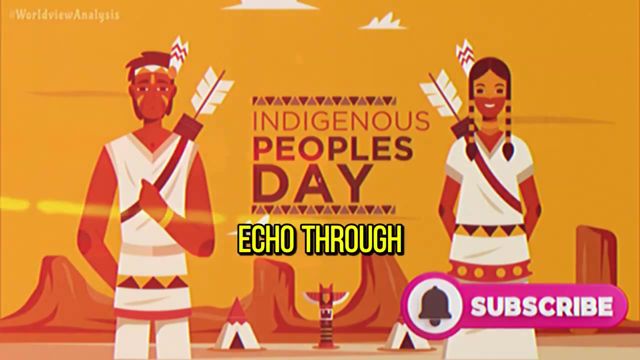 with silver, but also with fertile lands and abundant wildlife. The Spanish exploited these resources relentlessly, setting up large haciendas and forcing indigenous communities into servitude. This exploitation marked the beginning of a long history of economic inequality that would echo through the centuries. As the Spanish colonies grew, so did the disparities, The Spanish elite. 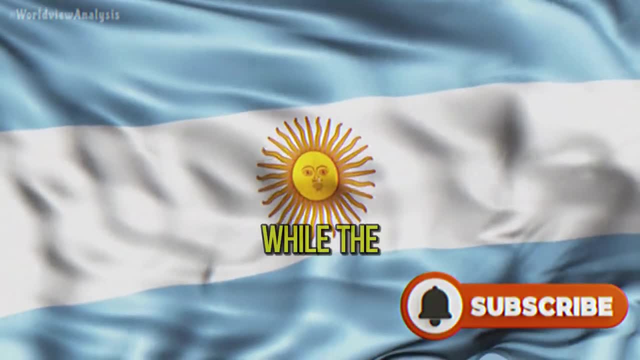 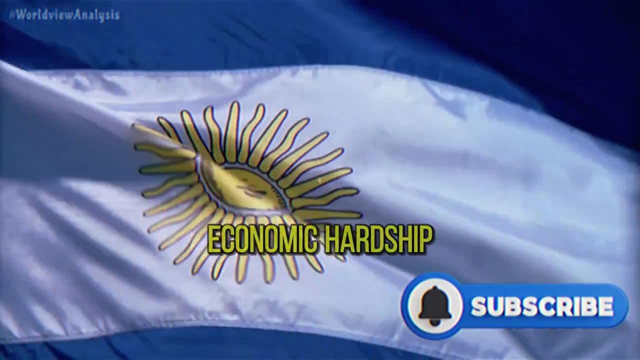 known as peninsulares, enjoyed a life of privilege, while the Creoles, those of Spanish descent born in the new world and the indigenous population bore the brunt of economic hardship. The social order was a stark reflection of the economic divide, with wealth concentrated in the hands. 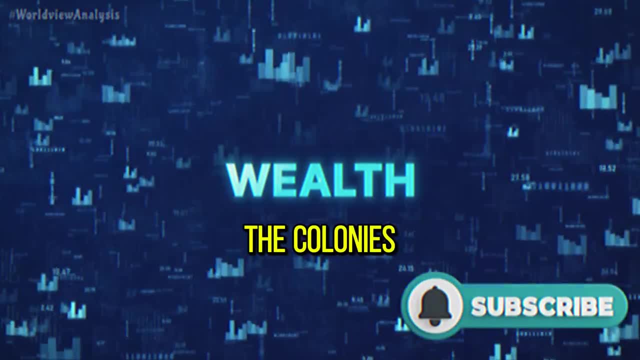 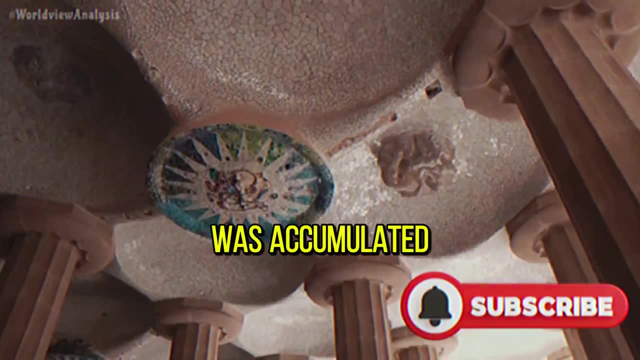 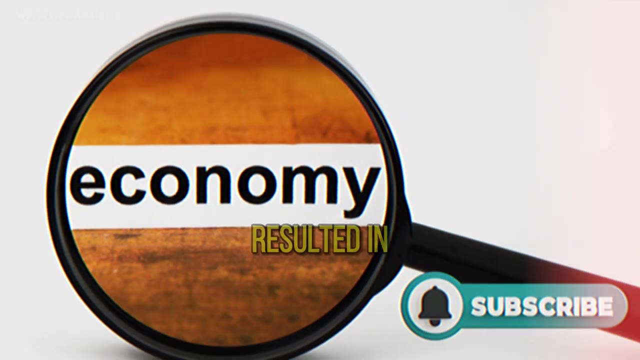 of the few. The economic structure of the colonies was designed to serve the interests of the Spanish crown. Resources were extracted, wealth was accumulated, but little was invested back into the local economy or the welfare of the people. this short-sighted approach resulted in a fragile 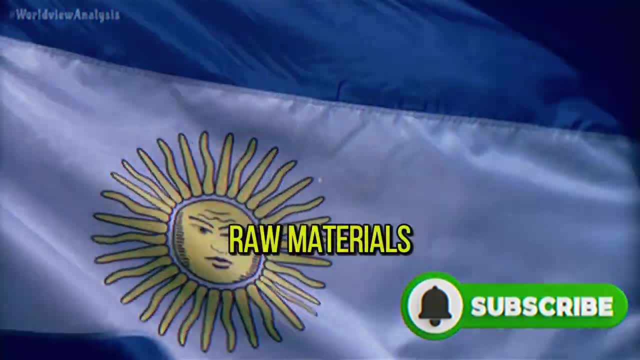 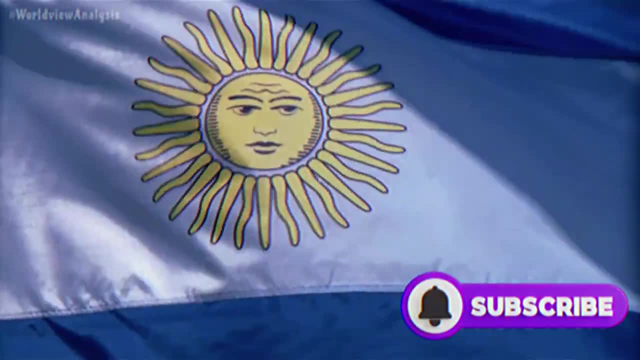 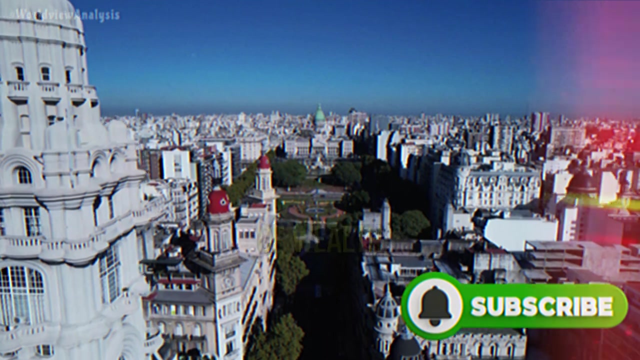 economy heavily dependent on the export of raw materials and vulnerable to external shocks. as we delve deeper into argentina's colonial past, we begin to see the underpinnings of its future economic challenges: the exploitation of labor and resources, the concentration of wealth, the lack of. 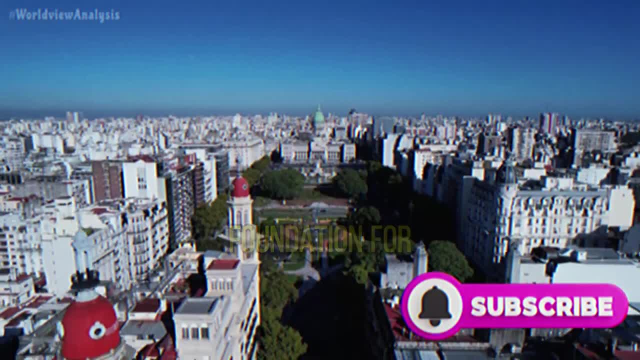 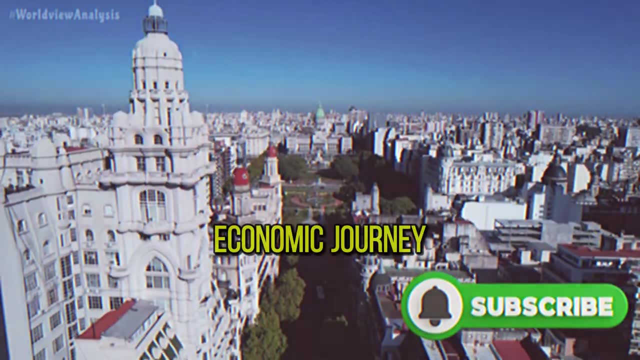 investment in the local economy. all these factors laid the foundation for the economic disparities that would persist into the modern era. so as we trace the arc of argentina's economic journey, it becomes clear that its colonial past played a pivotal role in shaping its economic present. and 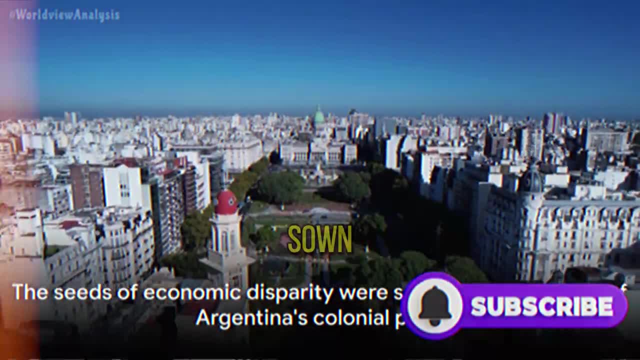 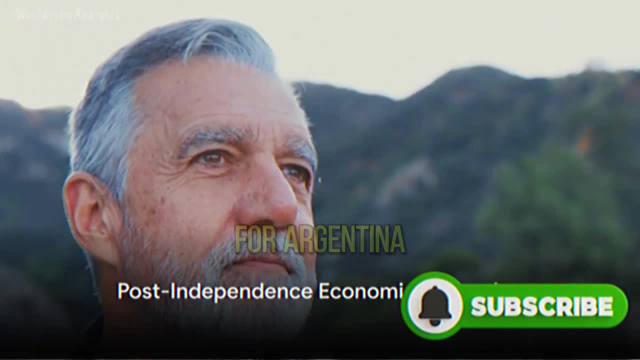 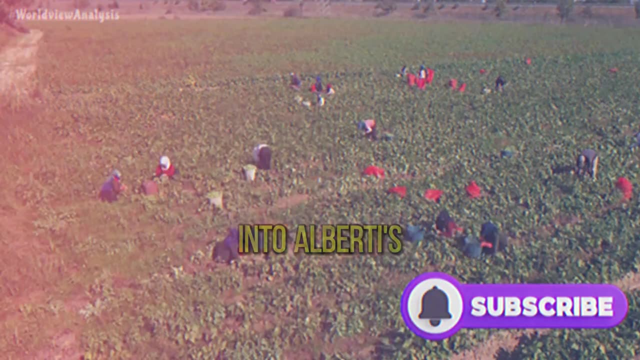 future. the seeds of economic disparity were sown deep in the soil of argentina's colonial past. independence brought new challenges and opportunities for argentina, and visionary leaders like juan batista alberti rose to the occasion. let's delve into alberti's economic strategies. 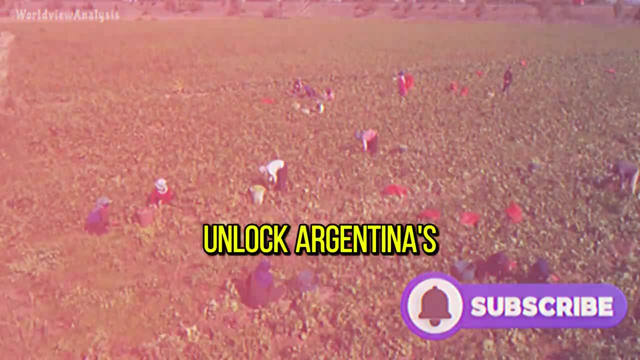 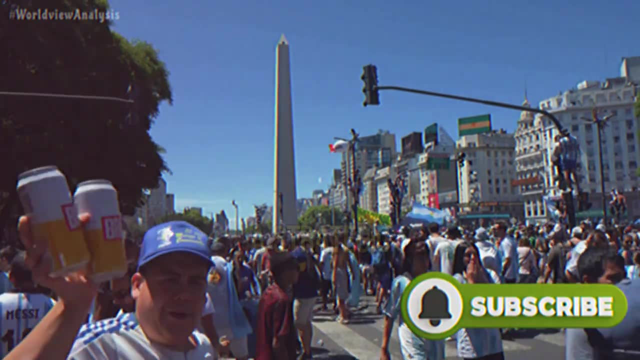 a man of foresight, alberti understood that to unlock argentina's potential, a fresh influx of labor was needed, so he set out to promote european migration. this was a strategic move, as the immigrants brought with them not just labor, but also a wealth of skills, knowledge. 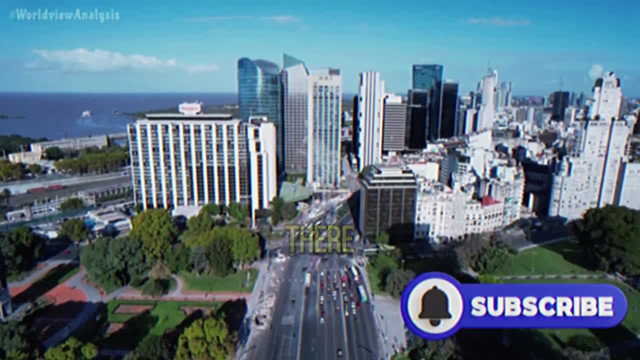 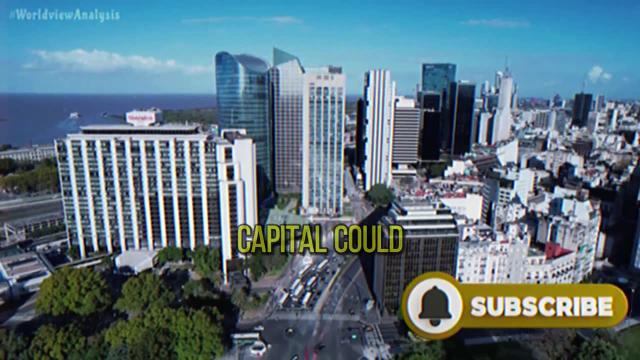 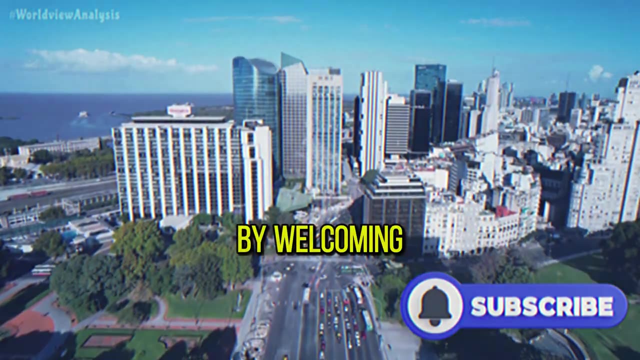 and cultural diversity. but alberti didn't stop there. recognizing the need for capital to fuel growth, he encouraged the development of new technologies, and the development of new technologies encouraged foreign investment. he knew that foreign capital could provide the resources necessary to build essential infrastructure and stimulate industrial growth by welcoming overseas. 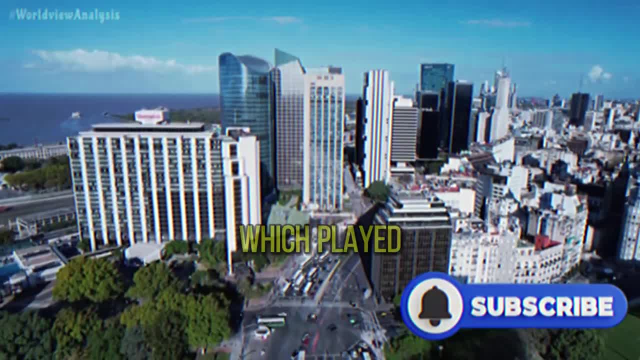 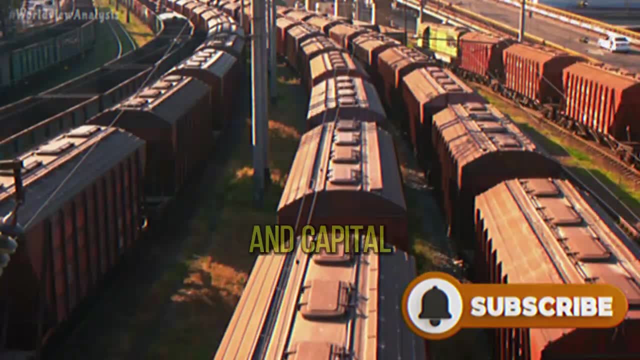 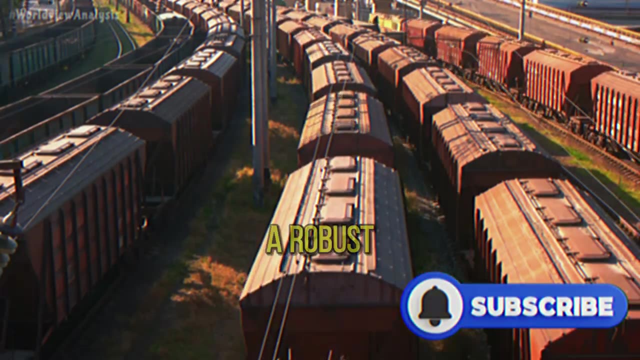 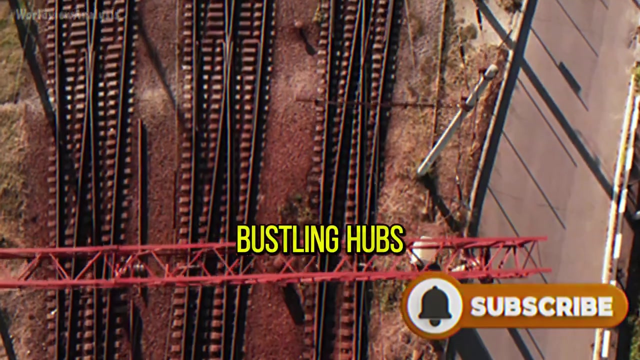 investors. he ensured the inflow of fresh capital, which played a pivotal role in argentina's economic expansion. alberti's strategies were not confined to people and capital alone. he also recognized the transformative power of technology, specifically the railroad. a robust railroad network was built to revolutionize argentina's economy. railroads could connect remote regions to the 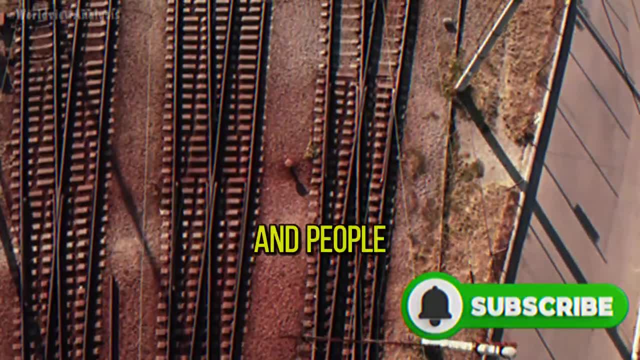 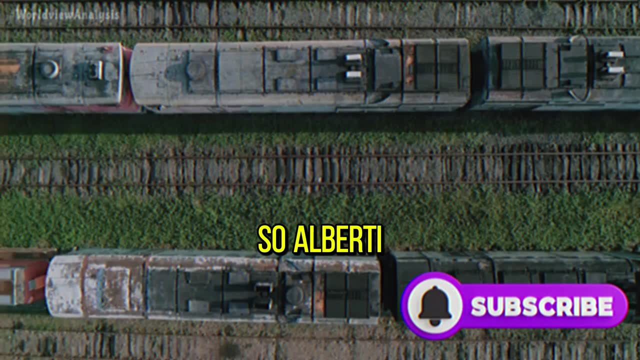 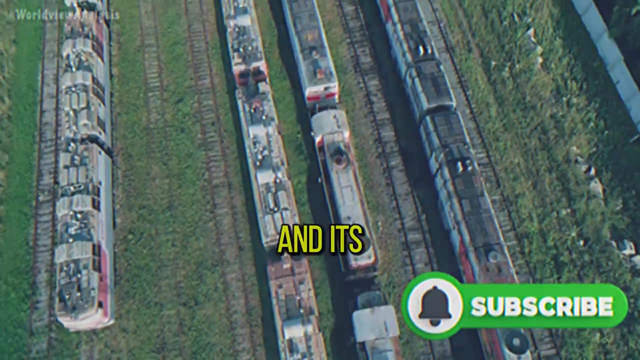 bustling hubs of activity and expedite the transport of goods and people. they could also open up untapped markets and create new economic opportunities. so alberti set out to build a comprehensive railroad network, a move that made argentina's vast landscapes more accessible and its resources more exploitable. this initiative not only addressed the issue of labor shortages, but 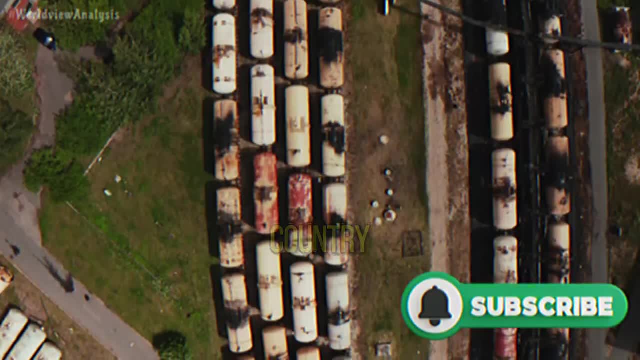 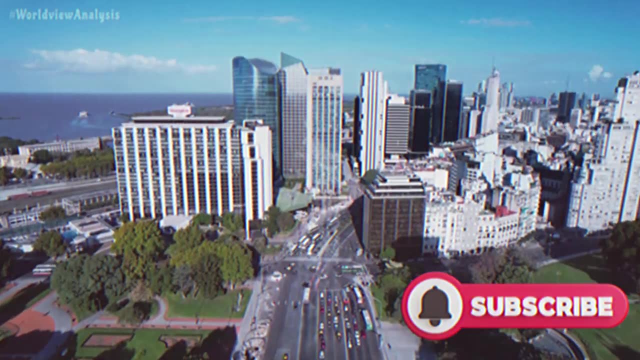 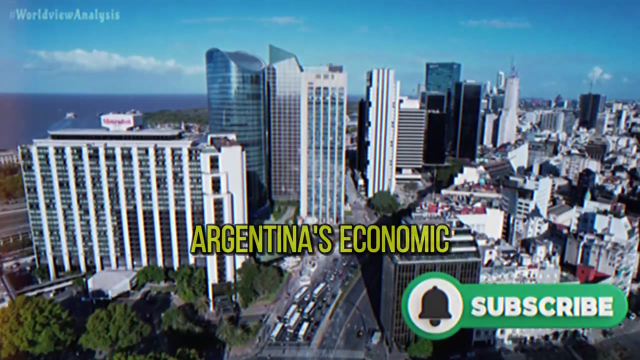 facilitated the easy movement of goods and services across the country, thereby boosting trade and commerce. alberti's strategies were bold and ambitious, but they were also based on a clear understanding of argentina's needs and potential. he knew that the key to unlocking argentina's 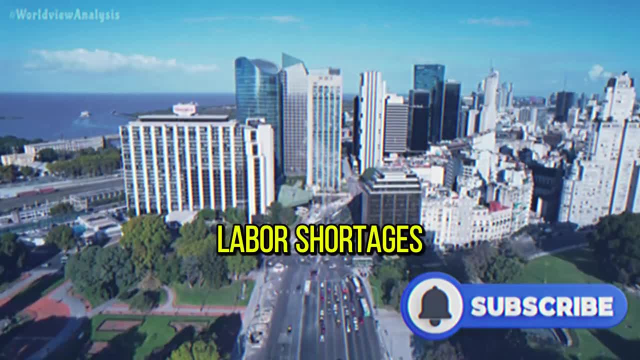 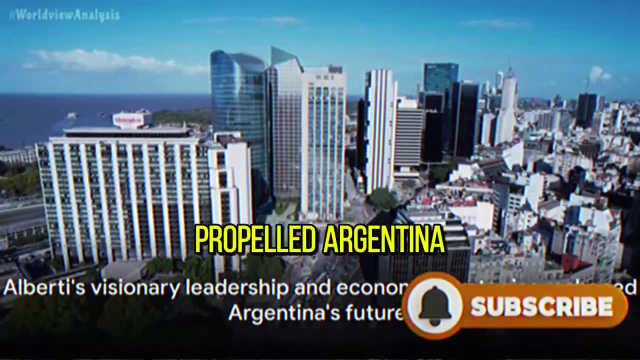 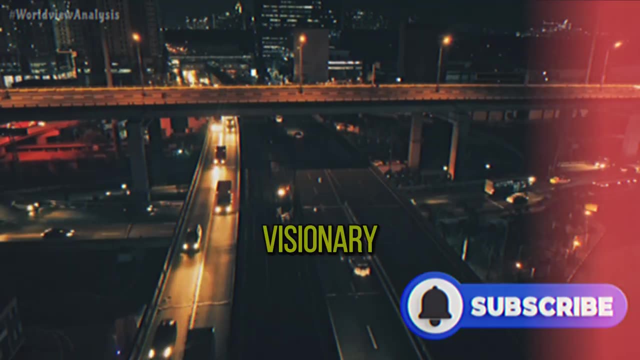 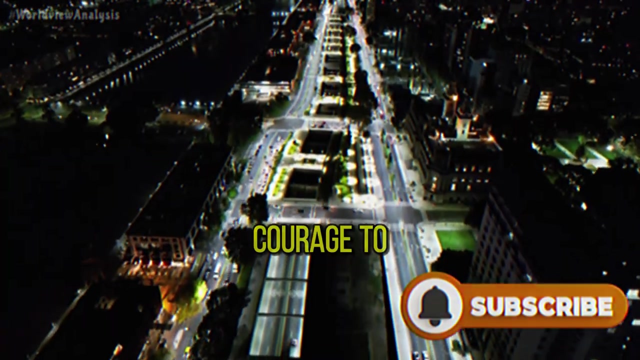 economic potential lay in addressing its labor shortages, attracting foreign capital and building a robust transportation infrastructure. alberti's vision propelled argentina into a new era of growth. his strategies stand as a testament to the power of visionary leadership in shaping a nation's economic destiny. they remind us that, with the right strategies and the courage to implement, 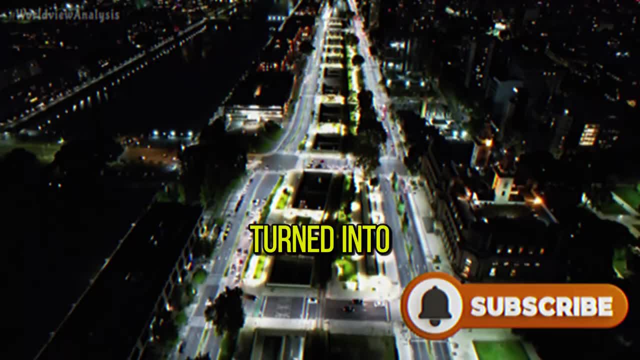 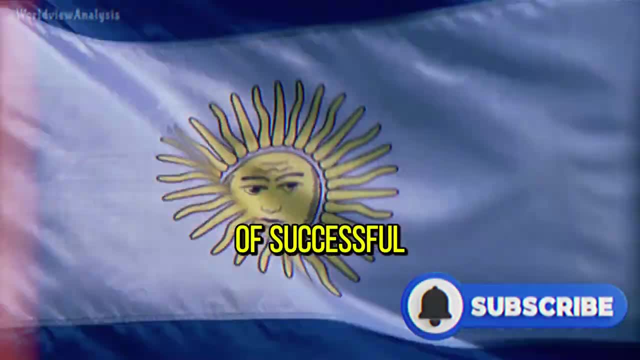 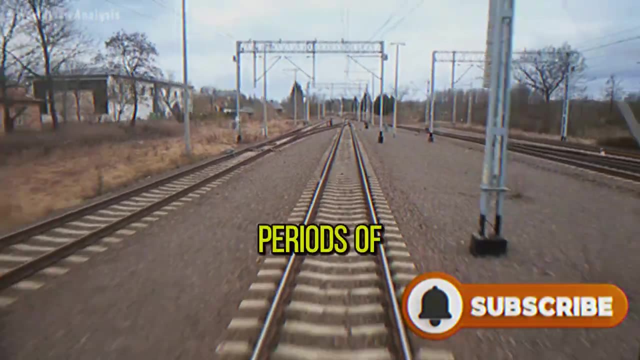 them. even the most daunting challenges can be turned into opportunities for growth and prosperity. political stability and strong leadership are often the bedrock of successful economies. argentina was no exception. the country's economic trajectory was significantly shaped by its economic growth and its economic growth in different periods of political stability. most notably under the leadership of general julio roca, serving as argentina's president in the late 19th century. roca was a strong leader who spearheaded policies that played a pivotal role in the country's economic growth. roca's tenure was marked by a consolidation of power. and an emphasis on the rule of law, providing the necessary stability for economic development. his government prioritized infrastructural development, notably the expansion of the railroad network, which connected argentina's vast territories and facilitated the movement of goods. this transportation revolution had a significant impact, stimulating trade and fostering economic growth. furthermore, roca's administration also embarked 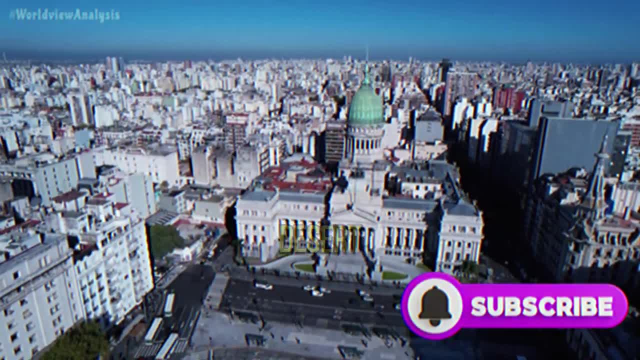 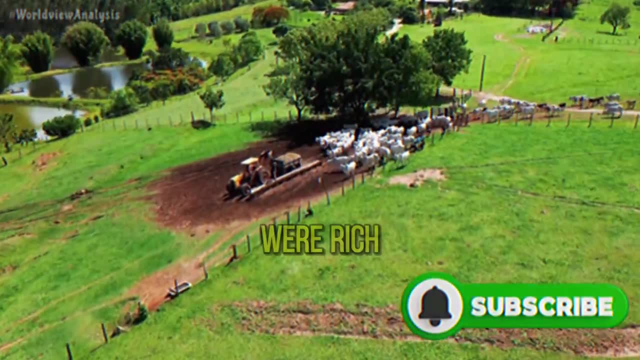 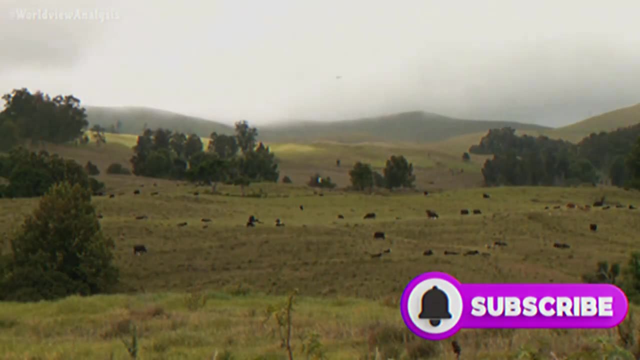 on military campaigns, often referred to as the conquest of the desert. these campaigns, while contentious, resulted in territorial expansion. the newly acquired lands were rich in resources and provided ample space for cattle farming, a major driver of argentina's economy at the time. yet the consolidation of power also had its pitfalls. while it fostered economic growth, 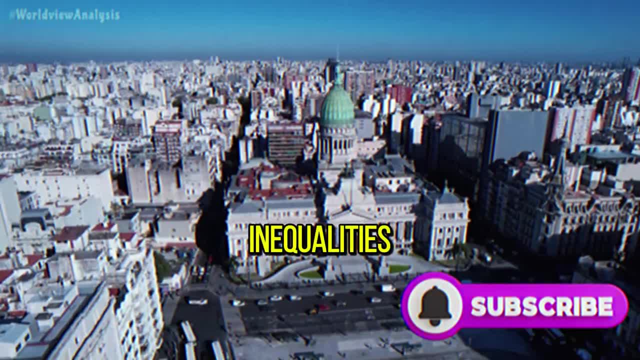 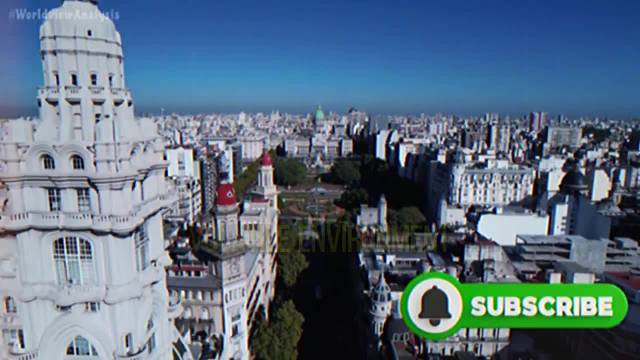 it also led to political exclusion and social inequalities. the concentration of wealth and power in the hands of a few, coupled with a lack of social inclusion, created a volatile environment that would later contribute to argentina's economic decline. moreover, the reliance on strong agricultural land and northern lands was soon lost, which led to an economic recession. 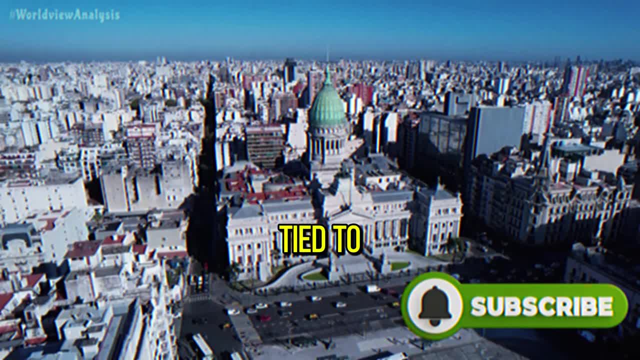 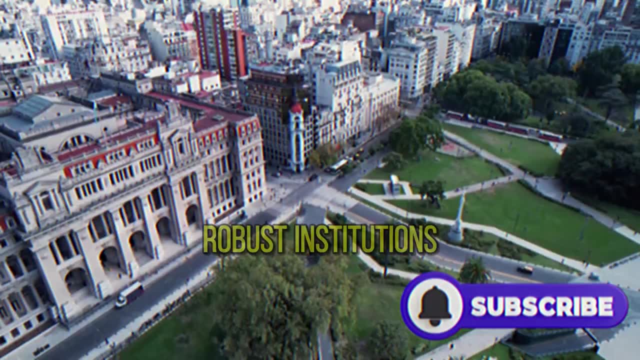 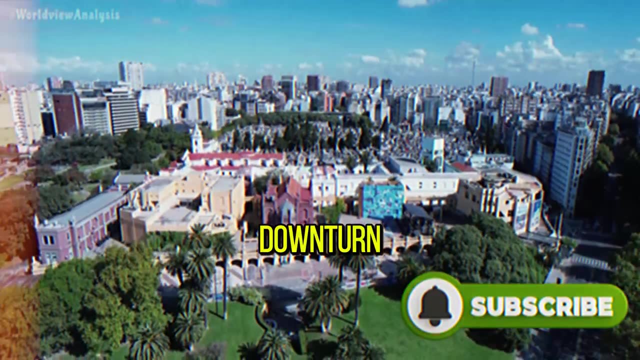 and conflict between the two countries. the conflict that suggested a strong economic. strong leadership meant that the economy was often tied to the whims and policies of the individual in power. This dependence on individual leaders, rather than robust institutions, made Argentina's economy vulnerable to fluctuations in leadership, contributing to its eventual downturn. 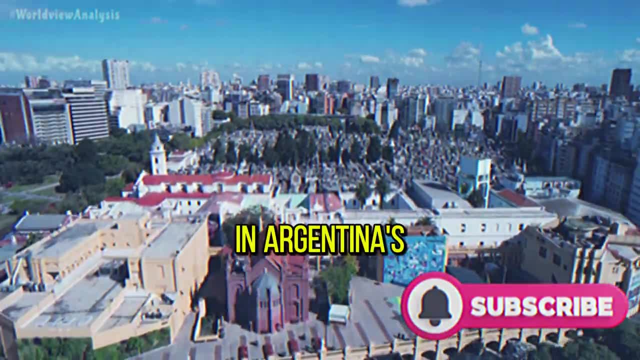 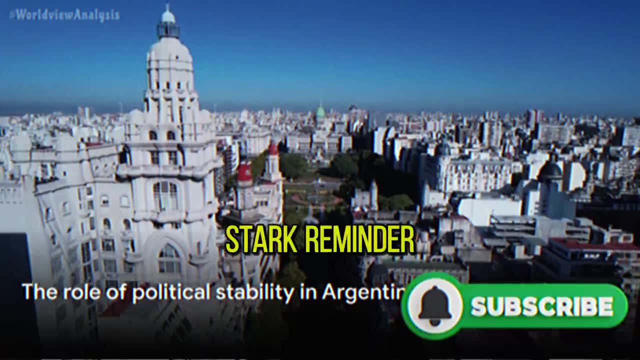 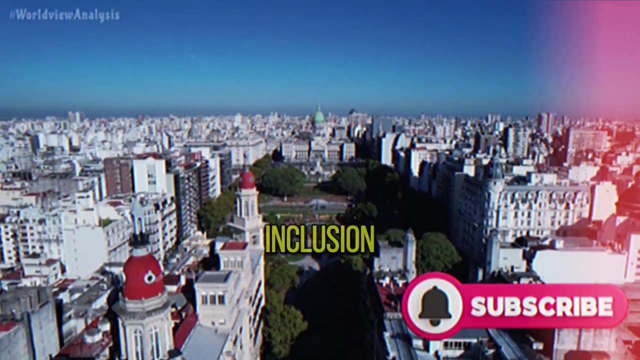 In essence, political stability played a crucial role in Argentina's economic ascent, but it was also instrumental in its downfall. The Argentine case serves as a stark reminder that, while strong leadership and political stability can foster economic growth, they must be balanced with social inclusion and 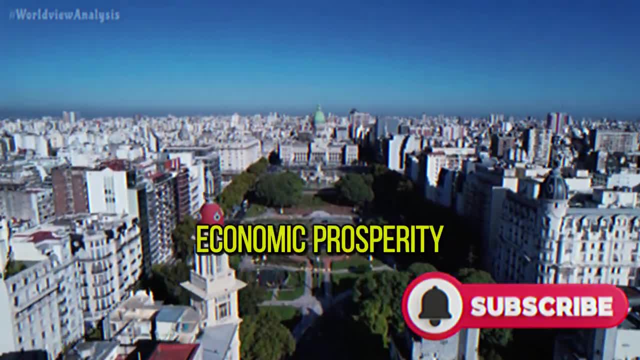 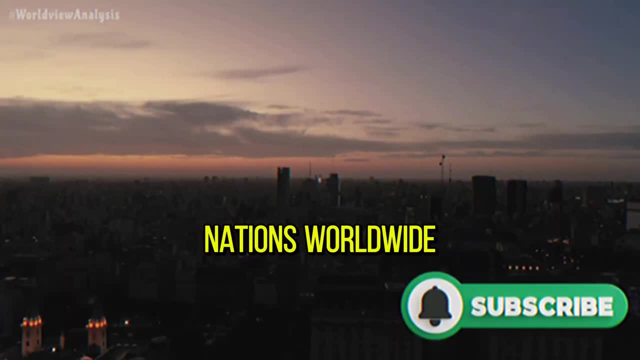 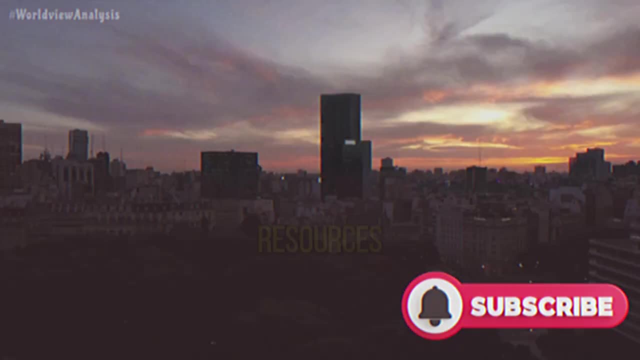 institutional resilience for sustainable economic prosperity. Argentina's rise and fall as an economic giant offers a wealth of lessons for nations worldwide. As we delve deeper into its economic journey, we find that the nation's prosperity was not just a product of its natural resources or geographic advantages. 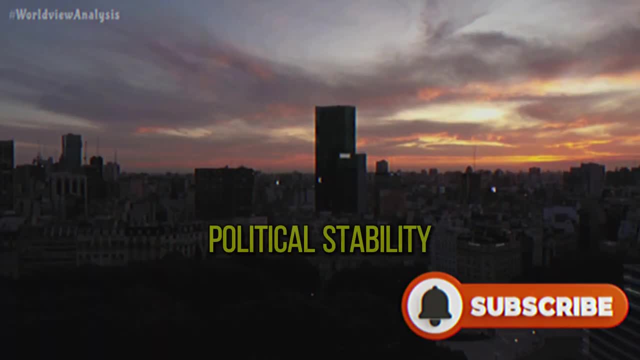 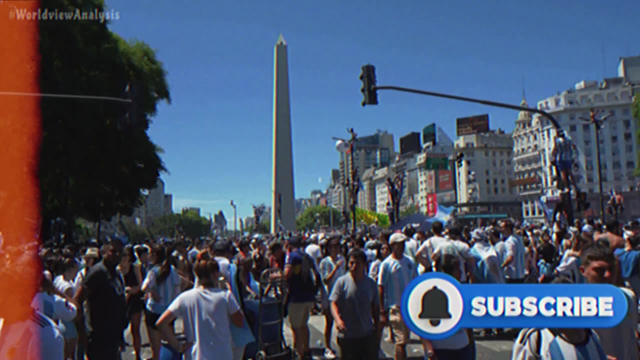 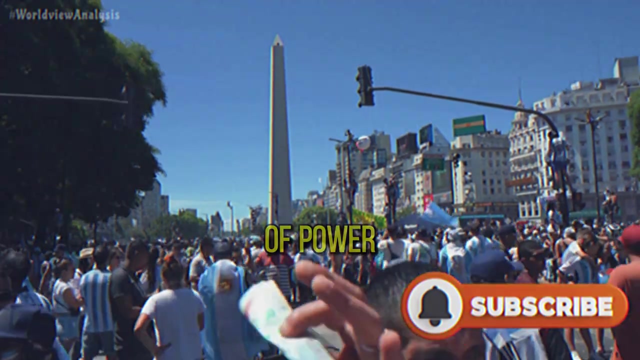 It was a product of its economic advantages. It was intricately linked to factors such as political stability, visionary economic planning and a persistent approach to addressing social inequalities. Political stability, for instance, played a crucial role in Argentina's economic growth. The consolidation of power under strong leadership, as seen during General Julio A Roca's 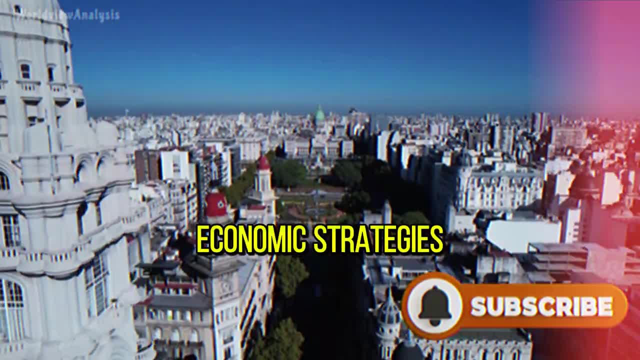 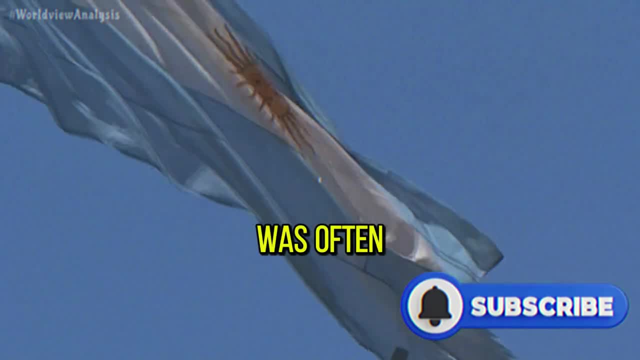 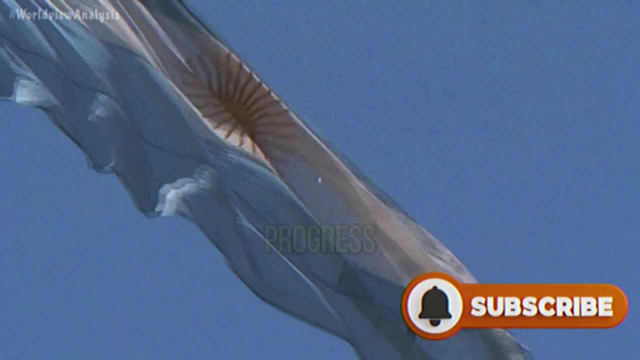 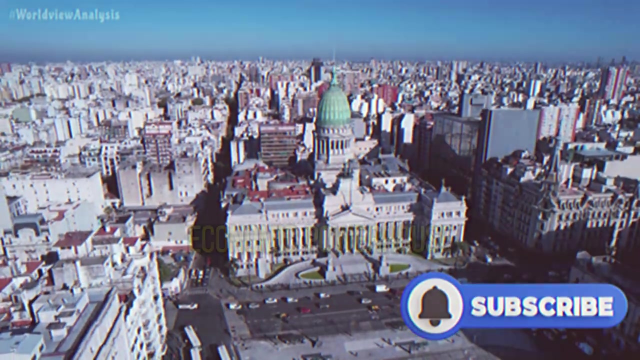 time facilitated the implementation of economic strategies and fostered an environment conducive to foreign investment and economic development. This stability, however, was often achieved through conflict and territorial expansion, demonstrating the delicate balance between political tactics and economic progress. Next, visionary economic planning was a driving force behind Argentina's rise as an economic 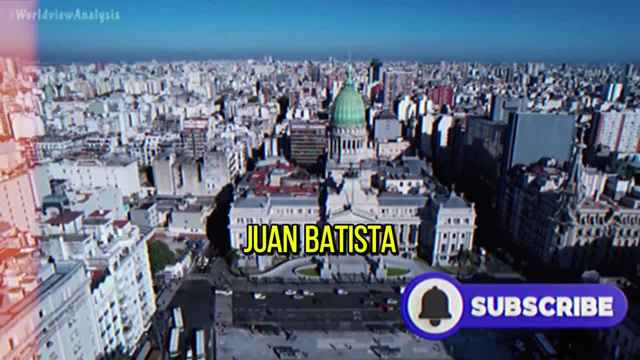 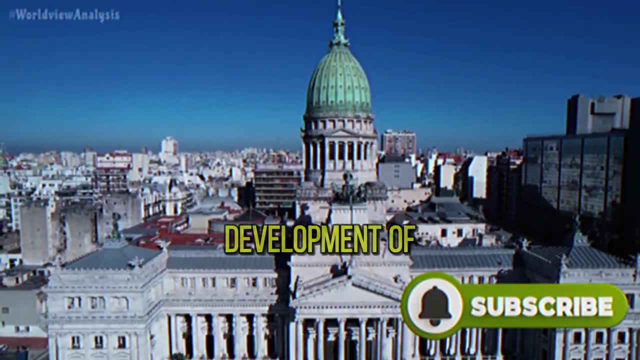 powerhouse. Take the example of Juan Batista Alberti's initiatives post-independence. His promotion of European migration, foreign investment and the development of a robust railroad network were deliberate strategies that helped him achieve his goals. These strategies aimed at addressing labor shortages and unlocking Argentina's economic 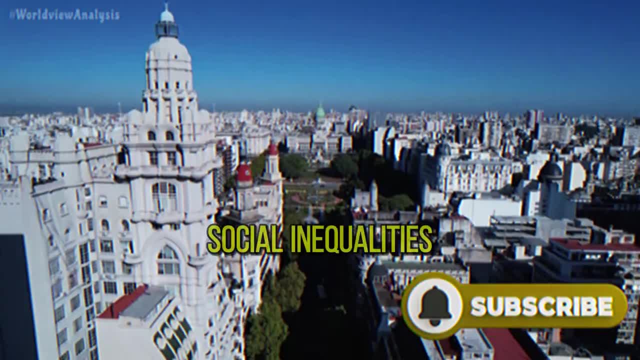 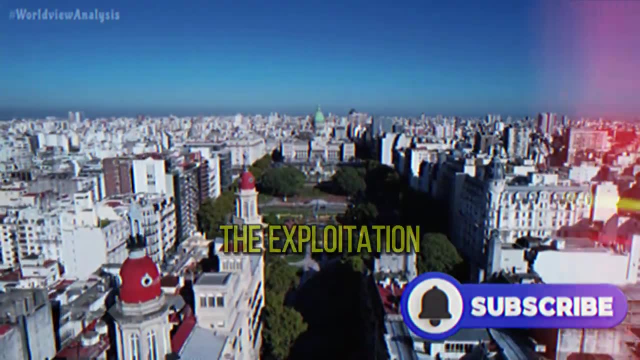 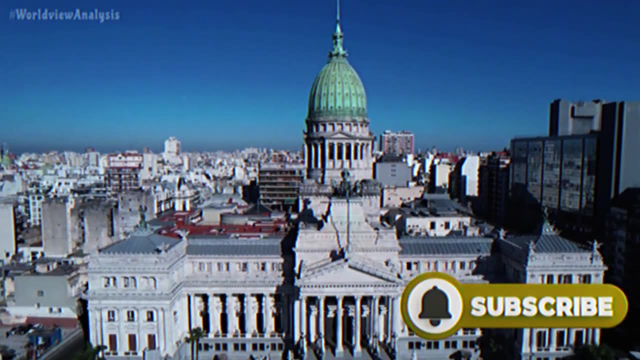 potential. Lastly, addressing social inequalities is crucial for sustainable economic growth. Argentina's colonial history, marked by the exploitation of labor and resources, sowed the seeds of economic disparities that persisted through the centuries. These inequalities have been a recurring challenge, underscoring the importance of inclusive growth. 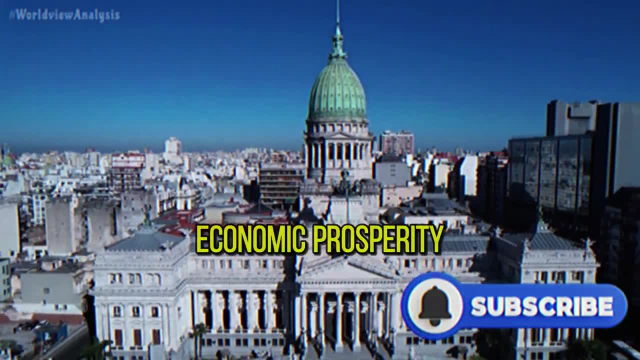 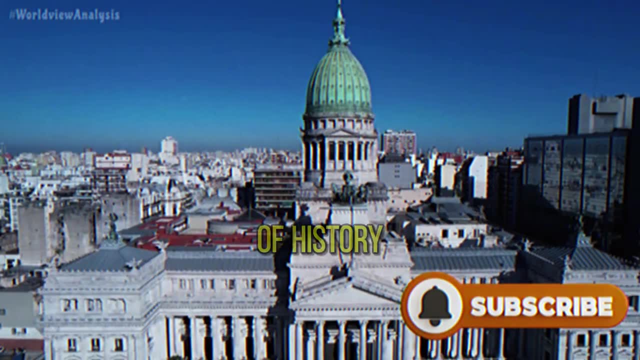 and equitable wealth distribution in maintaining economic prosperity. Argentina's journey from economic prosperity to decline is a testament to the complex interplay of history, politics and economics. It's a story that every nation striving for economic strength should heed.